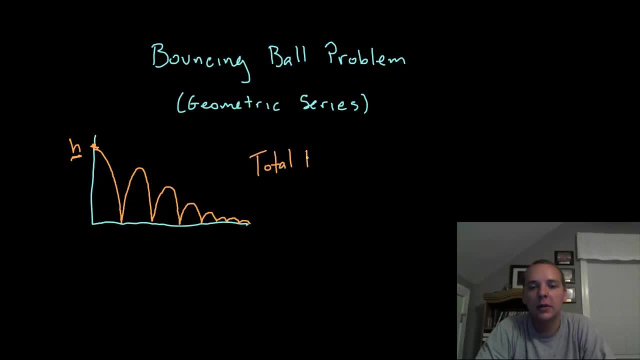 up. then what�s the total distance traveled, meaning the total vertical distance, not included with the horizontal distance, but the total vertical distance traveled. So in other words, if you had a slow motion camera and you were able to measure this initial height, you would take that distance, but then you would add back to it not only this distance here, that 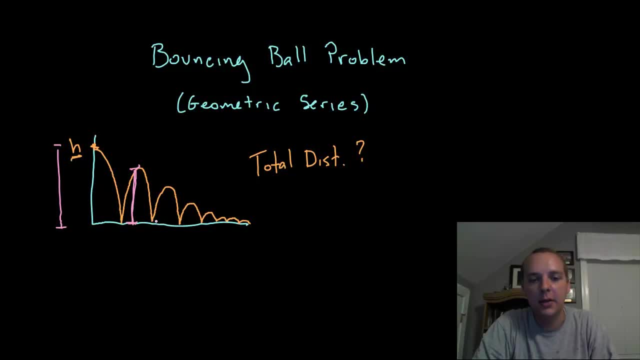 I�m showing, but actually twice that, because it goes up that much and then down that much again, and then two times this height plus two times this height, plus two times this height For forever, and it turns out to be a geometric series. so it gives a good application for. 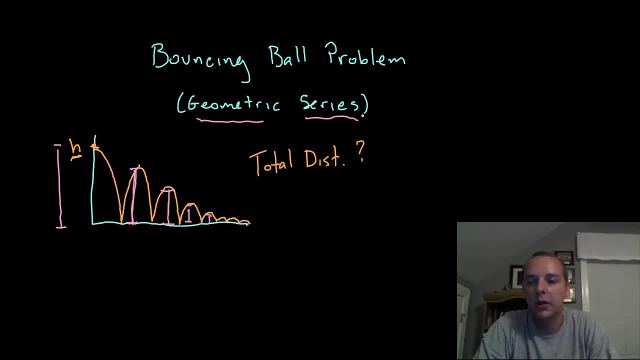 a geometric series. So let�s give one a shot. we�ll just make up some initial data and then we�ll see how it turns out. So let�s say our initial height, and you can change this to create another problem. but let�s say your initial height is, let�s. 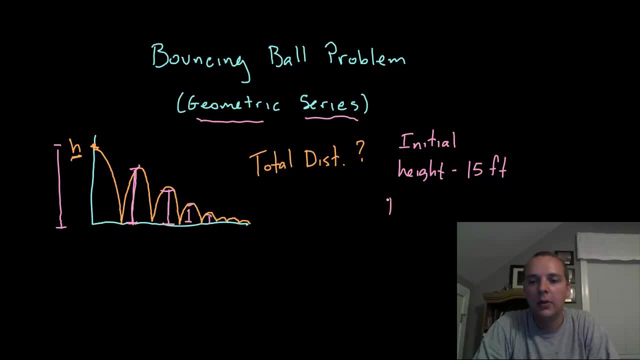 say 15 feet, And every time it bounces it will rebound. this may be given as a percentage or a fraction or a decimal, it doesn�t matter, Let�s say it will rebound. I�ll write it as a percentage: sixty percent of the way up. So if the initial height was hypothetically ten, then after the 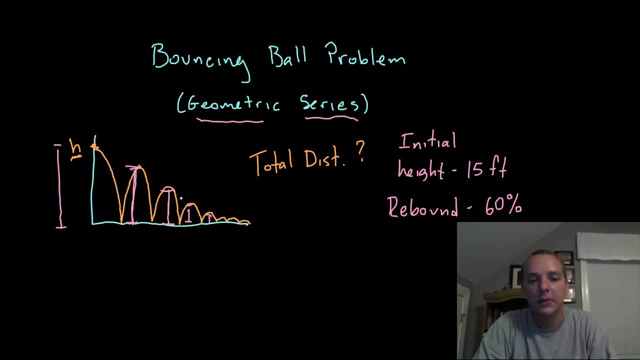 first bounce, it would only come up to a height of six, and then so on and so forth for every time below that. So let�s write this out, Let�s write this out long ways, and then we�ll take a look at how that turns into. 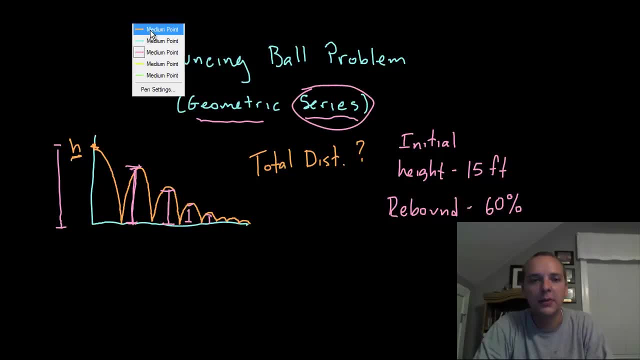 some sort of series. Let�s just write it term by term. So initial height is 15 feet, so the first bounce or the first drop would be 15, and then for the second height it will be sixty percent of 15.. So our 15 times six tenths, sixty percent of 15, but the second. 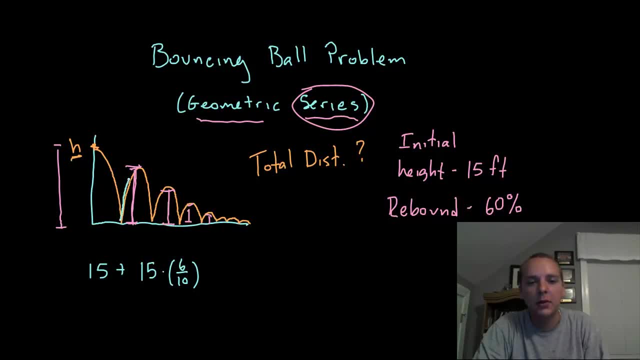 bounce after the first bounce is a little different than the initial drop because we go up and down. So I need to double this distance because, unlike the first drop, I actually have this distance traverse twice. And then after the second bounce, when you�re in this little interval here. well then, how? 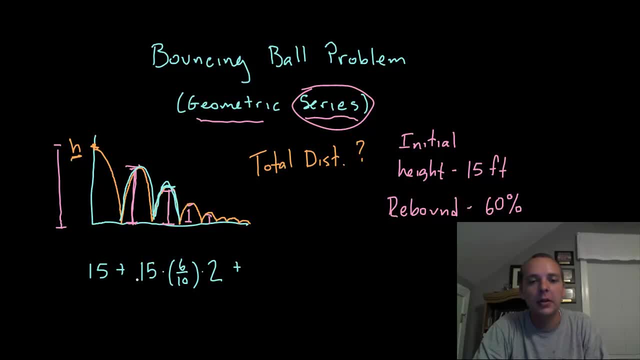 high is that? Well, the height will be sixty percent of this that I�m underlining right here. So that will be two. Okay, And then I�ll just put the two out front, since it�s up and down like the last one. 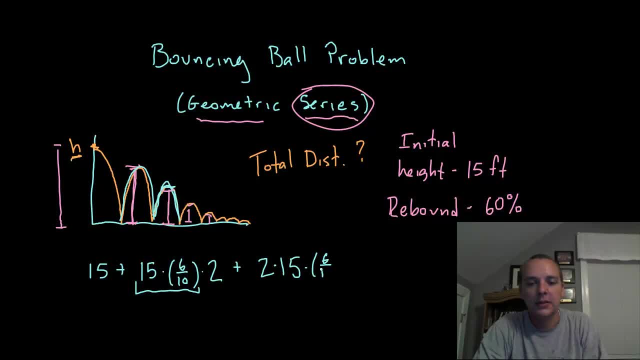 times 15 times six tenths, times another six tenths, sixty percent of that. so I�ll just write that as six tenths squared, And on and on and on. I think we see the pattern. then it will be two times 15 times six tenths. 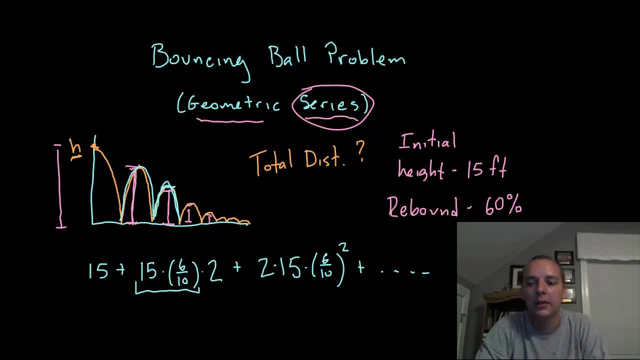 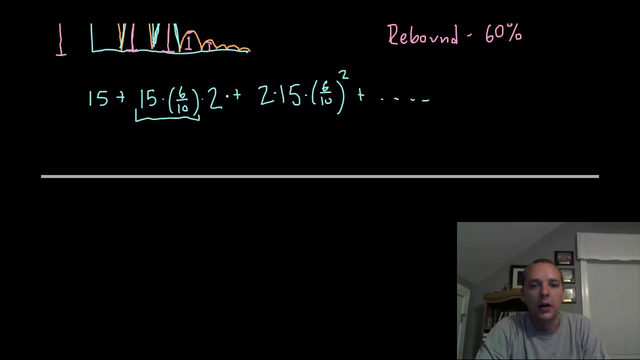 cubed, then to the fourth, then to the fifth, etc. So if we could figure out what this infinite series is, Then we�ll be able to tell the total distance traveled by the ball forever, until it comes to a complete stop. Alright, now, in trying to convert this into a series, one thing that we notice is going. 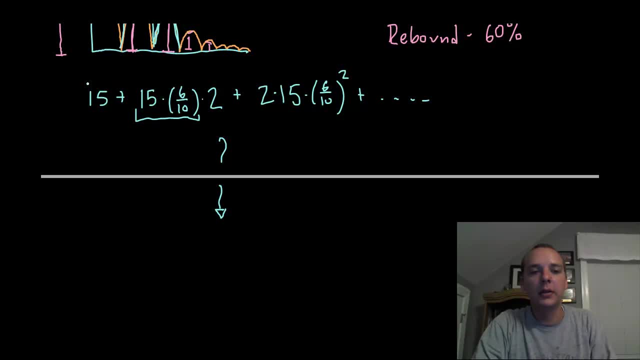 to be a little bit of a little bit of trouble, is this initial 15 out here. it�s not doubled, So what we�re going to have to do is break this apart into kind of two pieces. we�ll leave the 15 by itself. 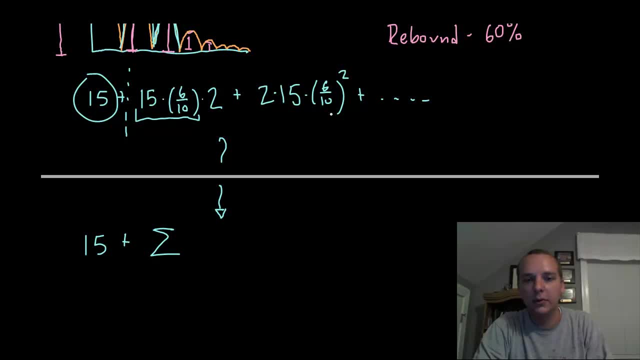 And then we�ll try to write the total distance traveled by the ball. Okay, Okay, Okay, Alright, so what we�ll be doing is we�ll be using the remainder of the rest of these terms as a series, So they all will have a two times 15, so all have a 30, but then the six tenths is what�s. 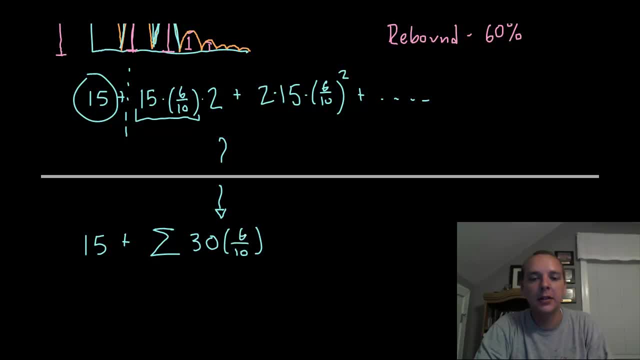 constantly increasing in power. so we�ll have six tenths to the nth power. first the first power, then the second, then the third, then the fourth, then the fifth, And notice, here n starts at one. six tenths to the first, the first term that you have. 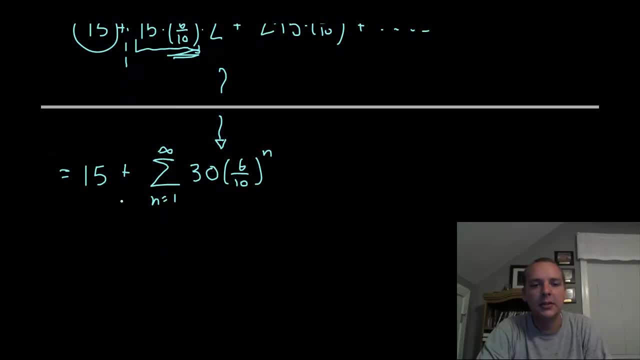 So this is looking pretty good so far. this is the same as this series here, plus 15.. If you look at the second term in the sum, this looks like a geometric series. almost just about the same as a geometric series, the only subtle difference hopefully you spotted. 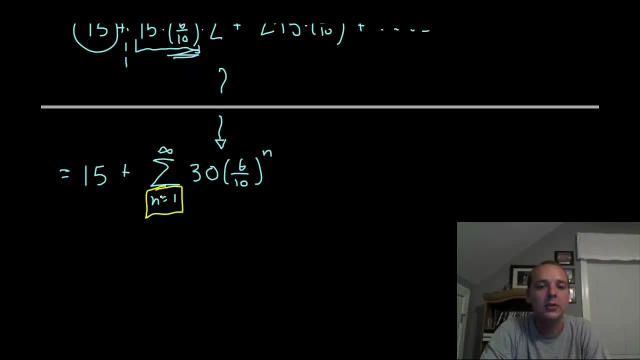 this is that it starts at 1, unfortunately, and it should start at 0.. Well, if you watch the video on geometric series, I talk about how to handle this discrepancy here, because there is a formula for the sum of a geometric series: you take A over 1 minus. 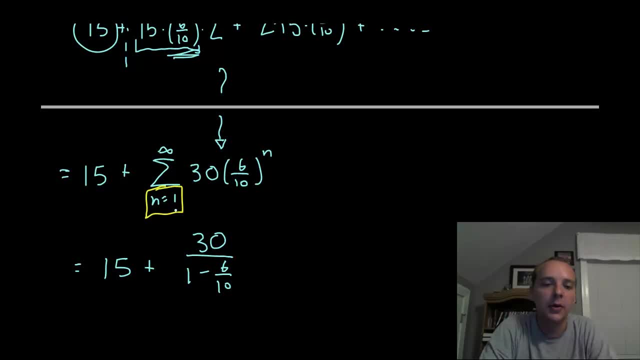 R, assuming that you�re starting at 0. So this is actually too much, because this formula here- A over 1 minus R- is for the full and complete geometric series that starts at 0. So how do I count for the missing term? because this is too large, I have the 0th term incorporated. 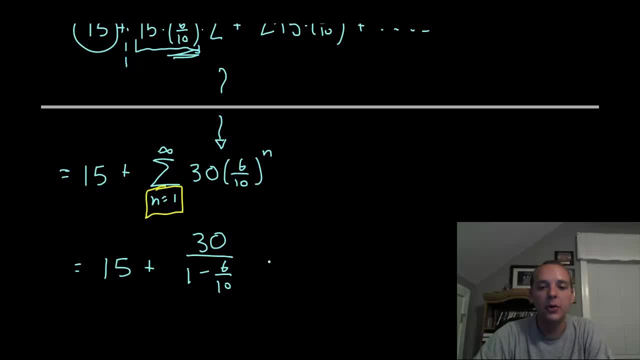 into this answer that shouldn�t really be there. it was very simple. I take this answer that is a little too large and I subtract out the extra term that should not have been in there. So if N was 0,, 30 times 6 tenths to the 0, power is 30 and I�m going to remove that. 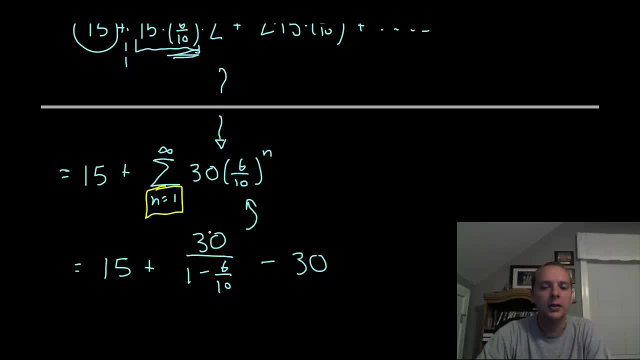 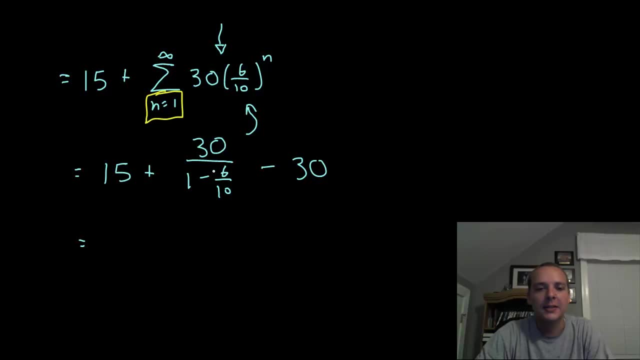 from the sum so that it really will be equal to this series right here. So just a little bit of algebra left. Let�s see 1 minus 6 tenths. 6 tenths will be 4 tenths, 4 tenths, 4 tenths times 30. I�m sorry, 30 divided by 4 tenths. 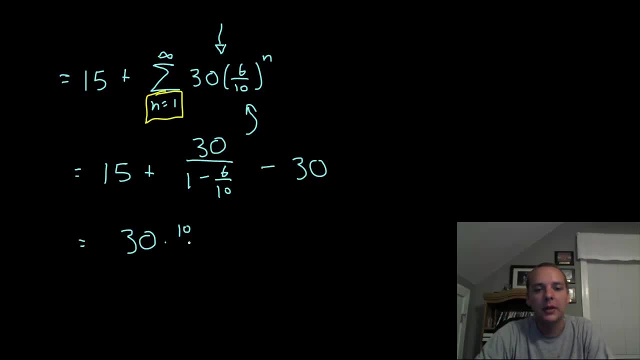 excuse me, we would have 30 times 10 over 4 if, instead of dividing by 4 tenths, you can multiply by the reciprocal. it�s a common algebra procedure. and then 15 minus 30 will give you minus 15, a little bit of algebra left. 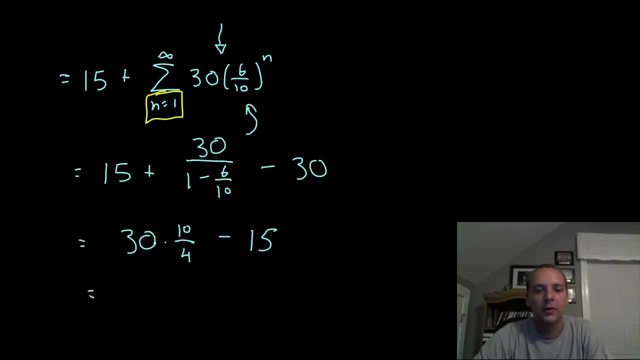 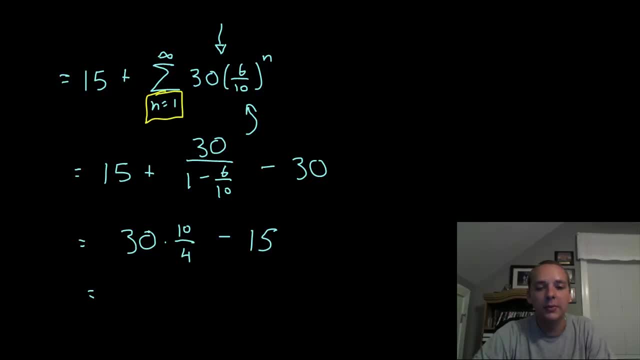 So 3 divided by 4 would be the same as 15 over 2, 15 over 2. it�ll reduce, but no more than that. You could make it a decimal if you wanted. 15 over 2 would be 7.5..